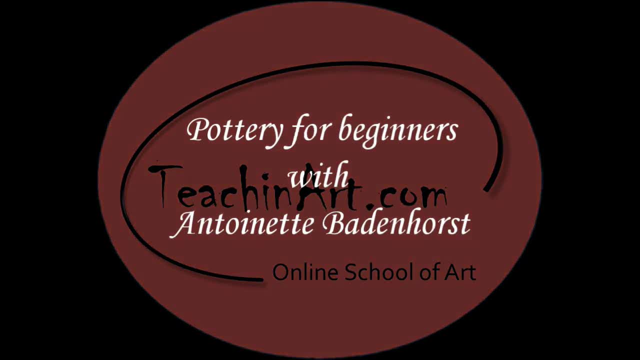 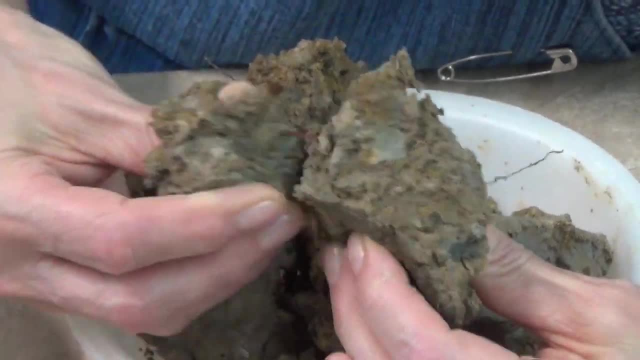 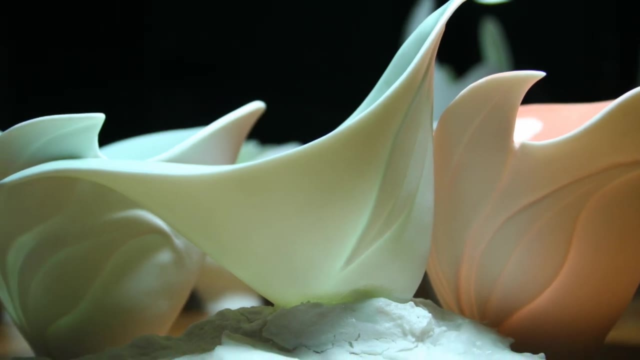 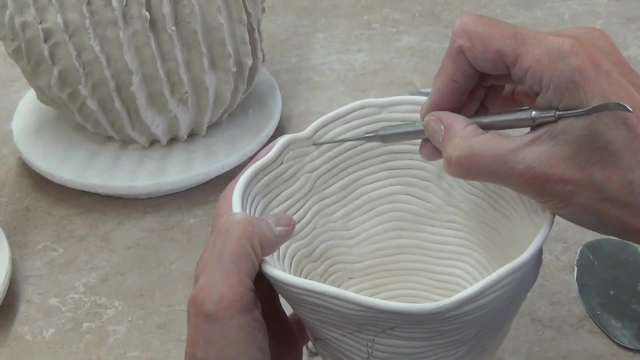 If you are watching this video, you are interested in getting to know where clay comes from and the process to when you have a finished product in your hand. I have been working in clay almost 40 years. I have taught many, many beginners from beginning, all the way to become professional. 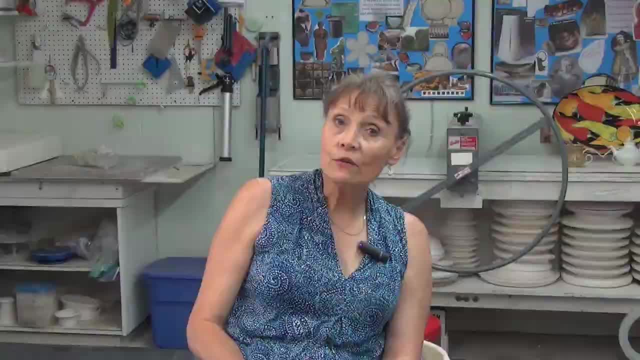 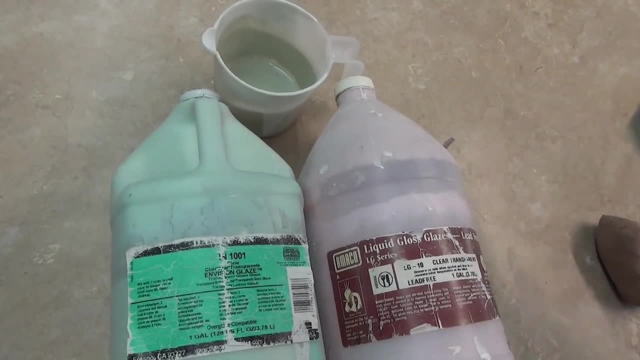 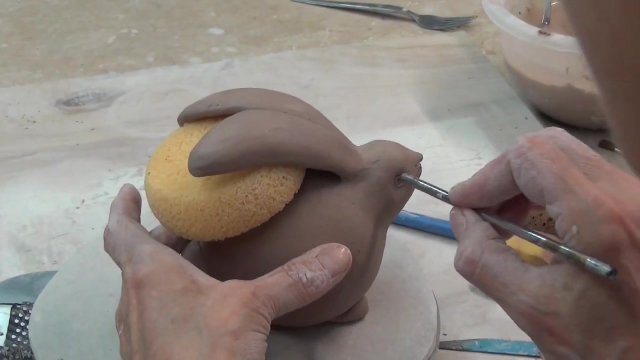 potters, When I am going to teach you, I'm going to give you the science behind the class, behind the clay that you're working with, behind the glazes that you're going to work with, so that you can understand exactly what you are doing. Various techniques. there's many of them There. 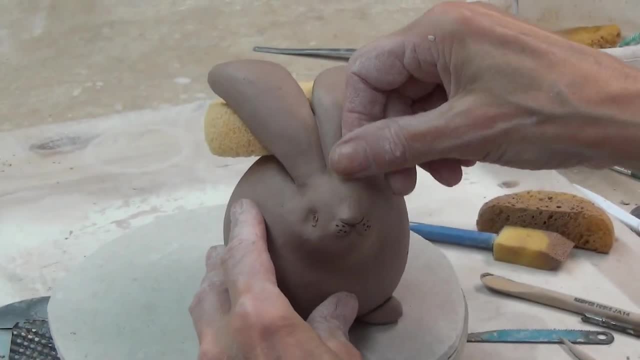 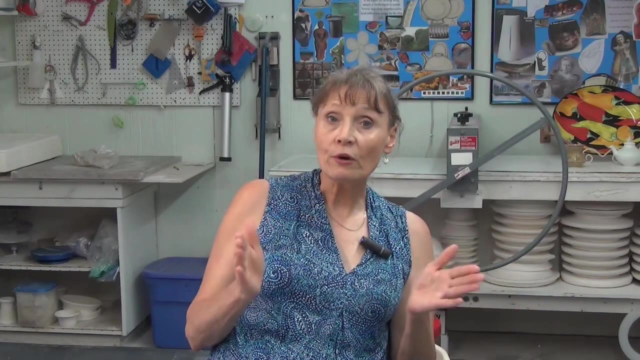 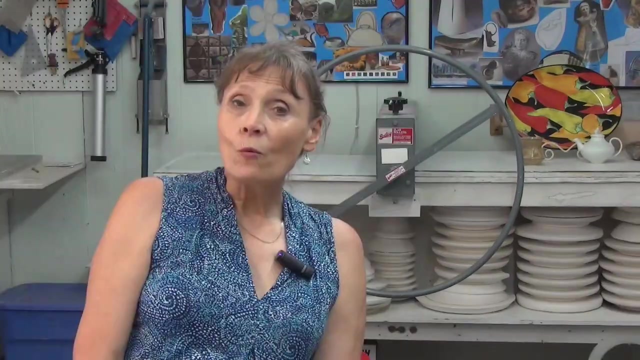 is no such thing as a one way or a way of perfection. There are many different ways to do what you are going to learn in pottery. The important thing is: you need to find the way that's going to work for you. What can you expect from me in this class? I've already mentioned to 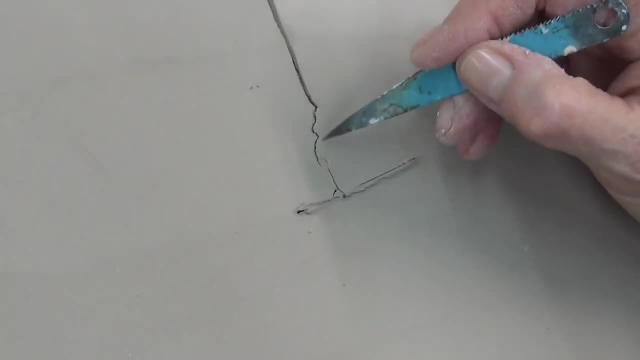 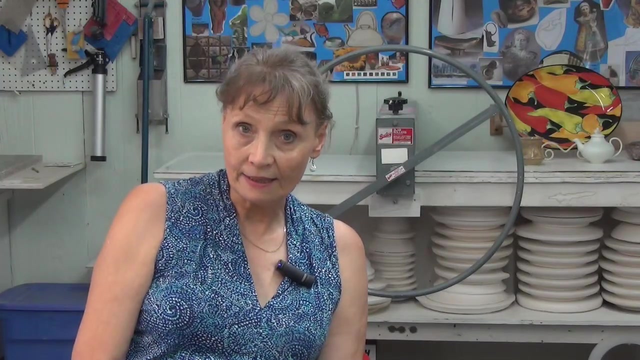 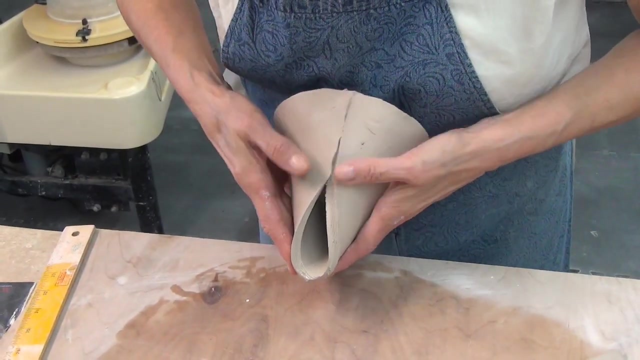 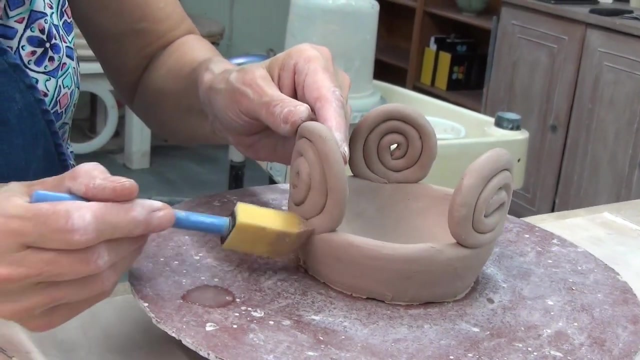 you that I'm going to give you some scientific background information. I'm also going to teach you some very basic beginner techniques, Starting out with simple pinching, going from there on to making a sheet or a slab of clay and making some coils. But before we do that, we need to find 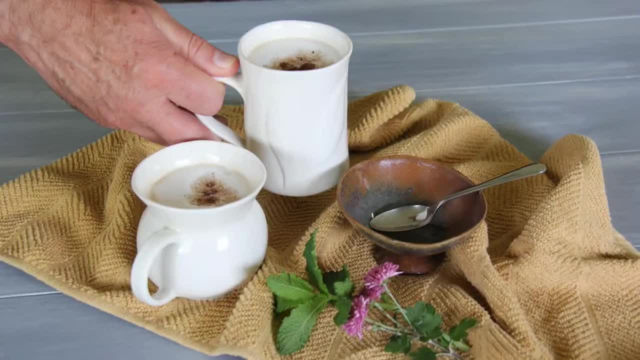 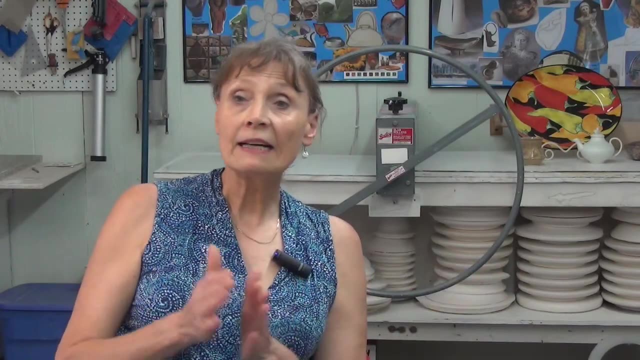 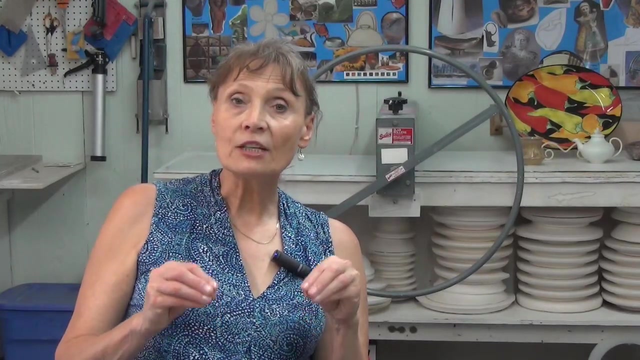 out if you are actually interested in pottery or if you're only interested in working with Fimo clay that people make jewelry from, clay that's been made in the kitchen from flour. If you're in a pottery class, it means that you want to make pots that's going to become permanent. 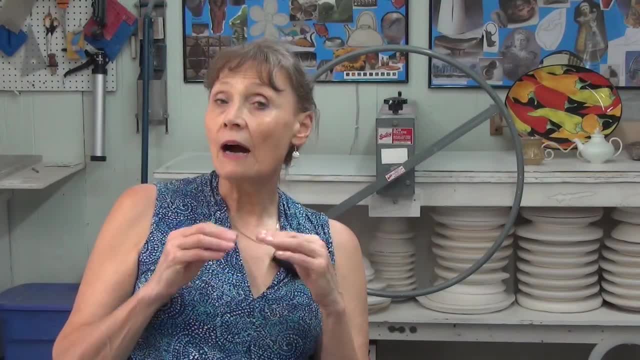 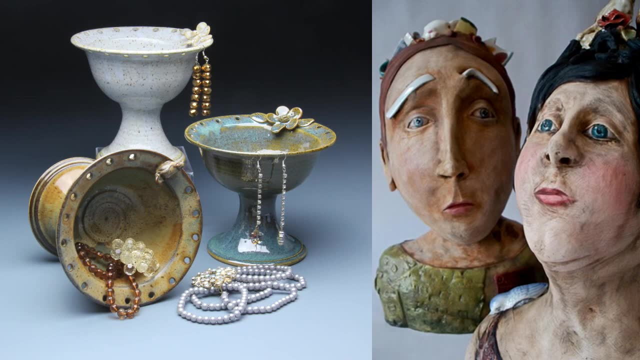 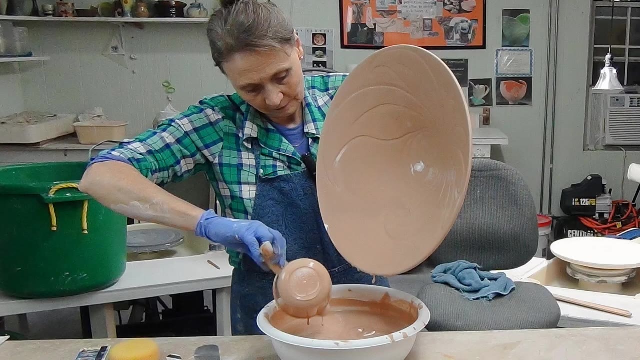 that you want to make objects that's going to be either ornamental- you can even do sculptural work while you're in this class- but you want to work with real earth. You will need access to a kiln, things like glazes. you can use paints on your stuff. You need clay.